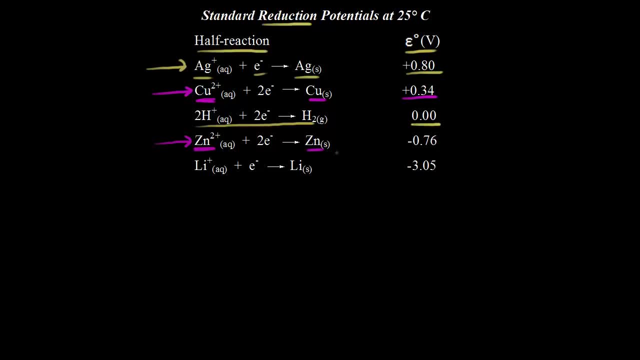 And if we are reducing zinc two plus to solid zinc, the standard reduction potential turns out to be negative 0.76 volts. The more positive value, the more likely the substance is to be reduced. So obviously positive 0.34 is more positive. 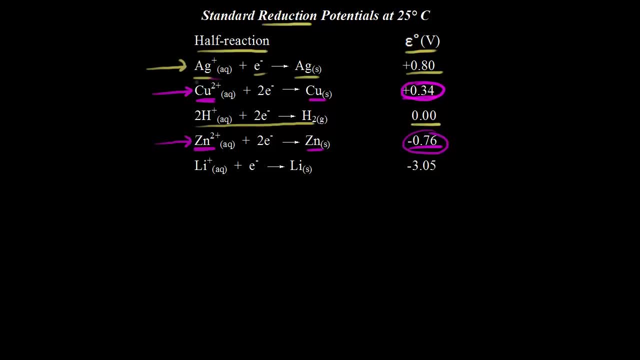 than negative 0.76.. So we know that this must be the reduction half reaction. So if we're talking about a redox reaction involving copper and zinc, this must be our reduction half reaction. So let's go ahead and write that. 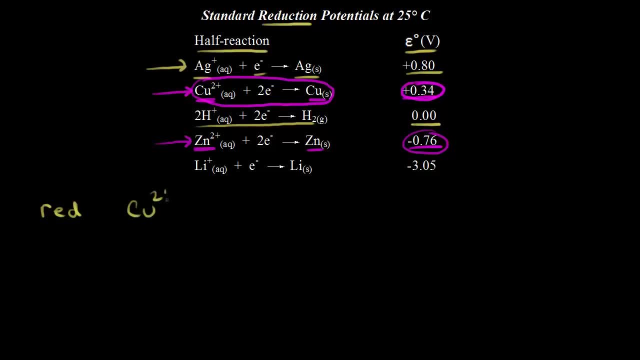 This is our reduction half reaction, where we have copper, two plus ions gaining two electrons to turn into solid copper And the standard reduction potential is positive 0.34 volts. So this is equal to positive 0.34 volts. Well, we know, in a redox reaction. 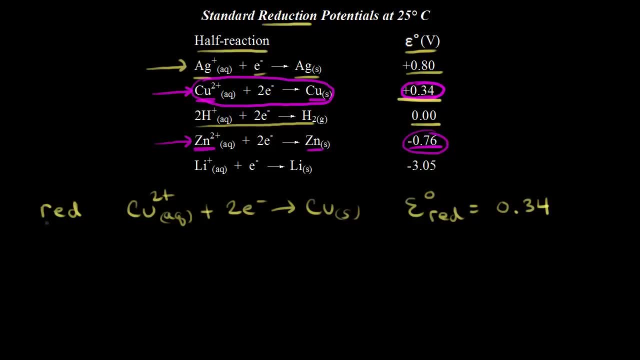 something is reduced and something is oxidized And since we already have our reduction half reaction, we need an oxidation half reaction. That must mean that this should be our oxidation half reaction, but here we have it written as a reduction half reaction. 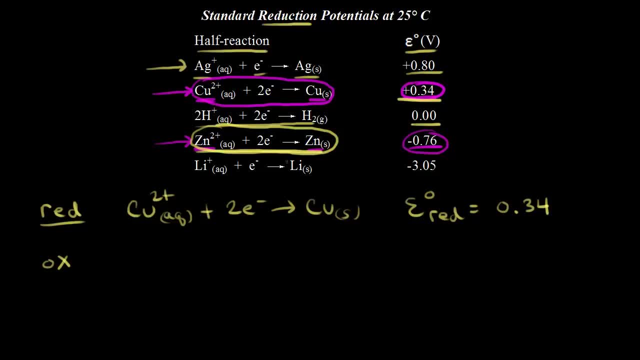 So we need to reverse this reaction to show it as an oxidation. We need to start with solid zinc on the left side. So we start with solid zinc on the left side and zinc is oxidized into zinc, two plus ions and we're losing two electrons. 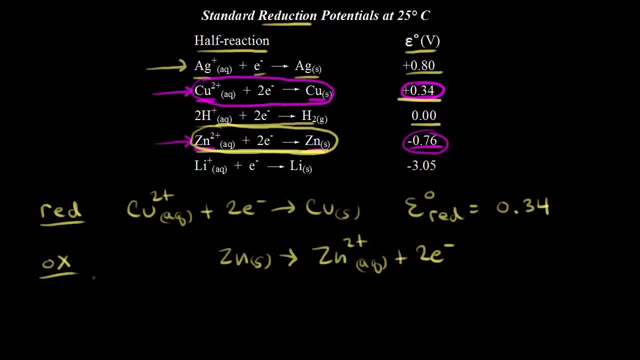 So, remember, loss of electrons is oxidation. So now this is an oxidation half reaction. So we need to find the standard oxidation potential for this half reaction And we can do that by looking at our table here. So negative 0.76 is the standard reduction potential. 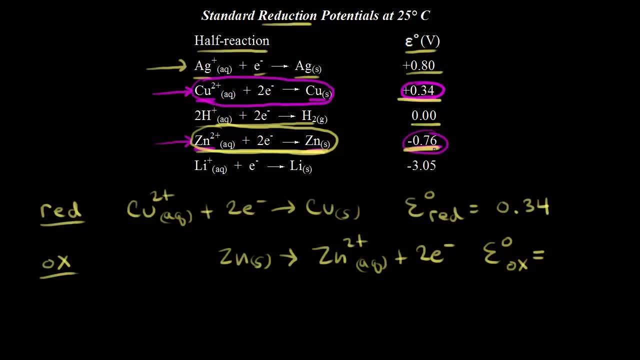 So since we reversed our half reaction, we just need to change the sign, So the oxidation potential must be positive 0.76.. So all we need to do is reverse the sign to get our standard oxidation potential, So we get positive 0.76.. 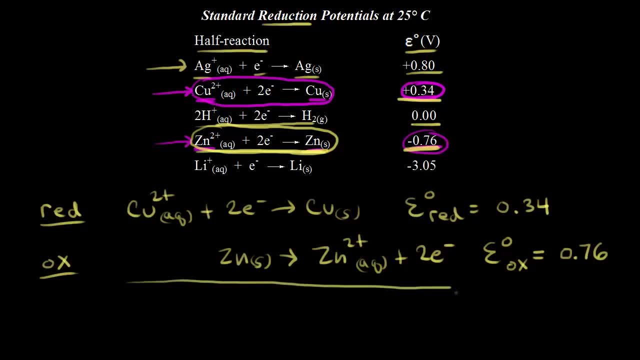 To find our overall redox reaction we just need to add together our two half reactions So to find our overall redox reaction. here we add the reduction half reaction and the oxidation half reaction. So these electrons would cancel out And on the left side we would get copper two plus ions. 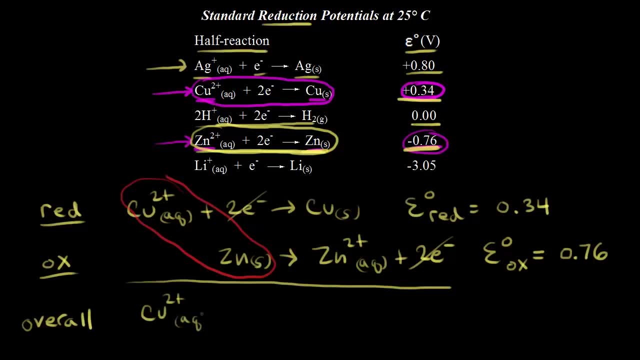 So this would be copper two plus ions and solid zinc, And on the right side for our products we would get solid copper and zinc two plus ions. So we get solid copper and zinc two plus ions. This overall redox reaction should look very familiar to you. 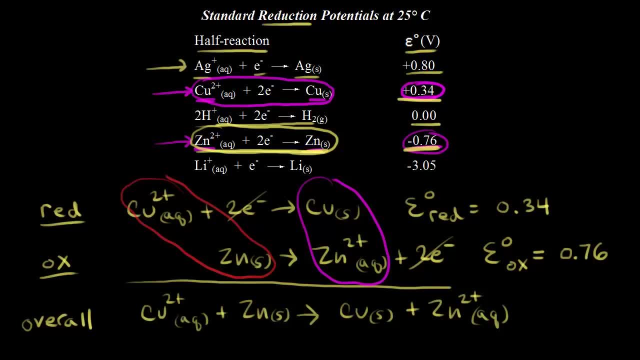 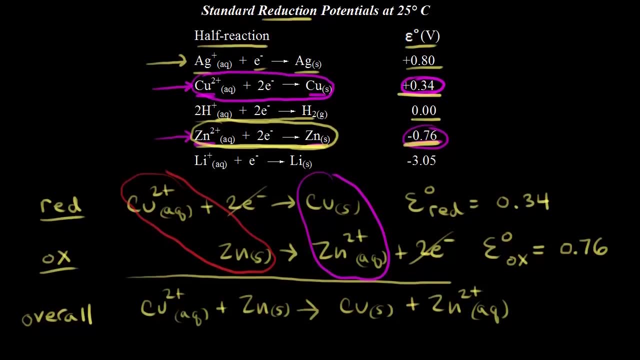 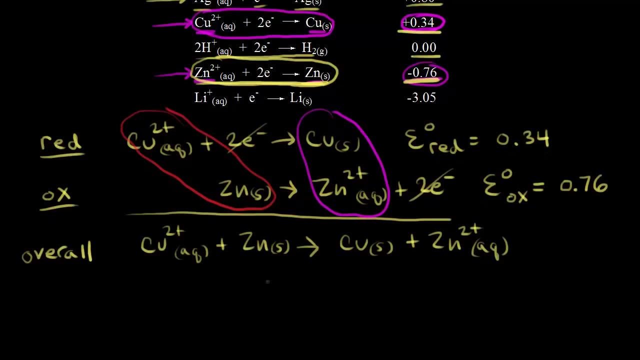 because this is the spontaneous redox reaction that we've talked about in the last several videos as our example of a voltaic cell. So we know this is a spontaneous reaction And how do we find the potential for the cell? All right, So how do we find the standard cell potential? 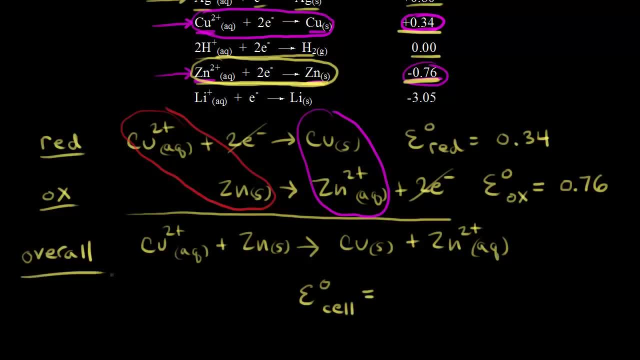 How do we find the potential for the entire cell? Well, to find the overall reaction, we add together our reduction half reaction and our oxidation half reaction. So that gave us our overall reaction. So to find our standard cell potential, we just need to add together our reduction potential. 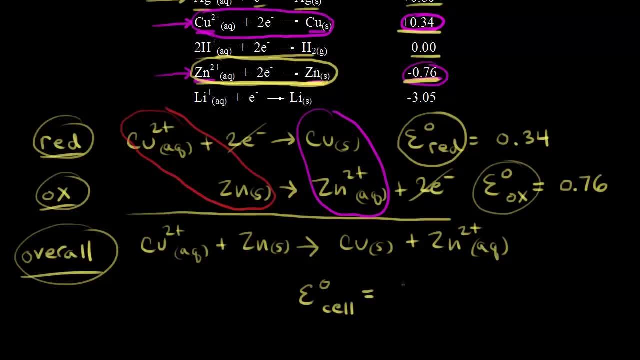 for the half reaction and the oxidation potential for the oxidation half reaction. So to find the potential for the cell, we add the reduction potential and the oxidation potential And so we get. when we do that we're going to get positive. 0.34 volts is the potential. 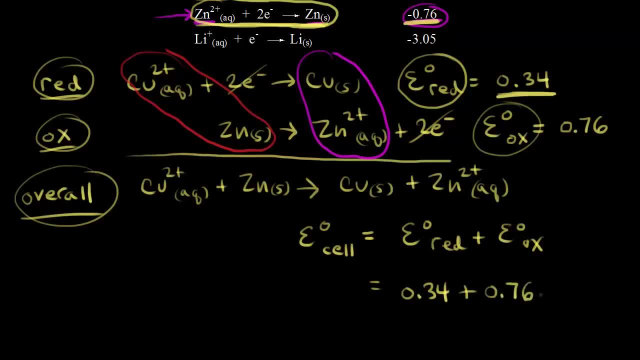 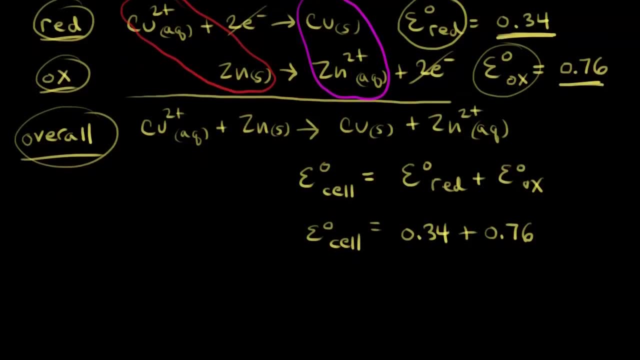 for the reduction half reaction, And positive 0.76 volts is the potential for the oxidation half reaction. So that gives us our standard cell potential. So for our cell the potential is equal to positive 1.10 volts, Which we already know. this from previous videos, right? 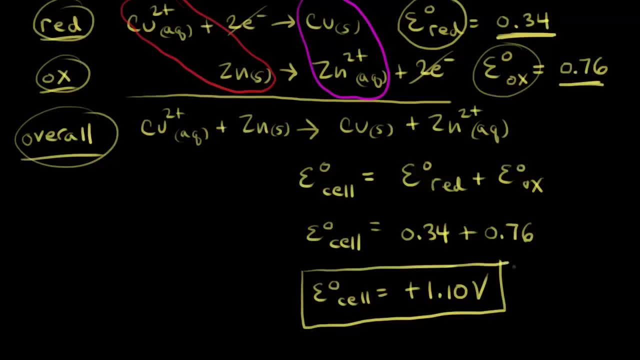 I talked about the fact that you could use a volt meter to measure the potential difference, to measure the voltage of a voltaic cell, And you're going to get positive 1.10 volts under standard conditions, And so that's one of the nice things. 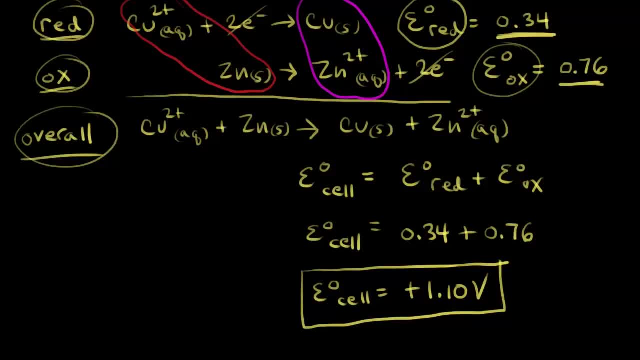 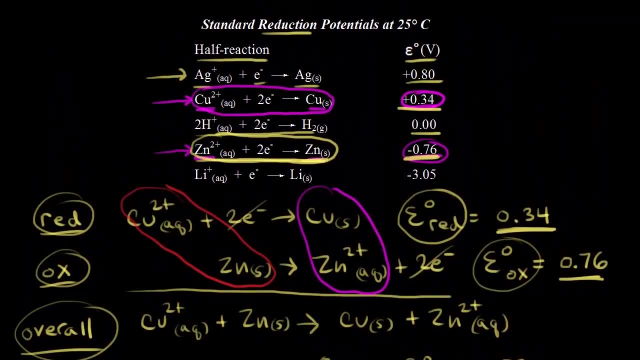 about the standard reduction potential table. We can calculate the voltage of our voltaic cells this way. Let's look in more detail at our half reactions. So let's start with the oxidation half reaction. We know that zinc is being oxidized, right? 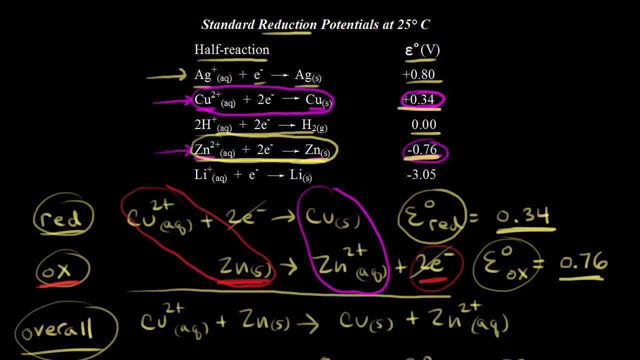 Zinc is losing two electrons And those two electrons that zinc loses are the same two electrons that cause the reduction of copper. So zinc is the agent for the reduction of copper. So we say that zinc is the reducing agent, And sometimes students find this confusing. 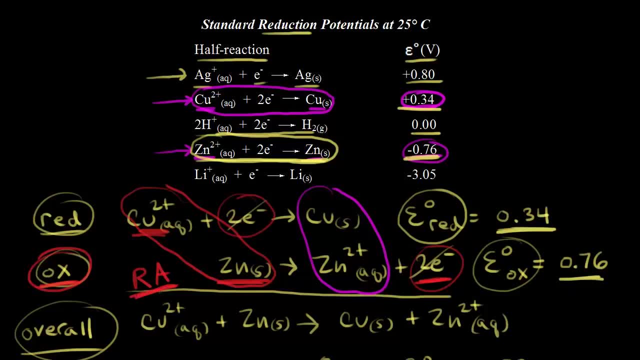 because zinc is being oxidized. So why is it the reducing agent? Well, zinc is the agent for the reduction of something else, In this case copper two plus ions. So zinc is the reducing agent. Copper two plus is gaining those two electrons. 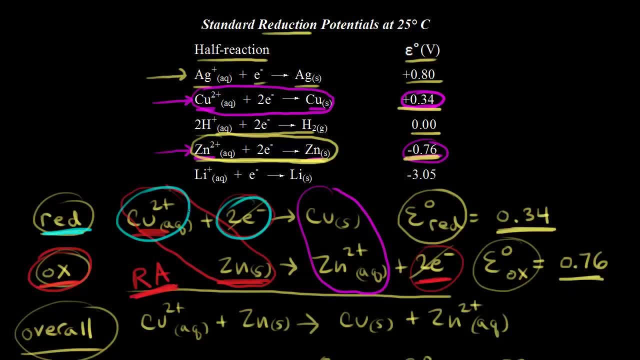 So copper two plus is being reduced. But because copper two plus is gaining those two electrons, it allows zinc to be oxidized. So copper two plus is the agent for the oxidation of zinc. So copper two plus is our oxidizing agent for our redox reaction. 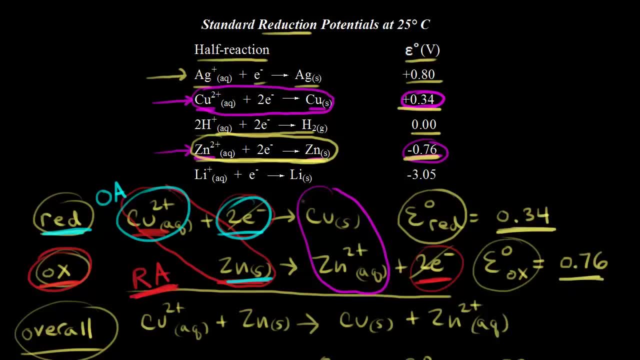 So let's look at our standard reduction potential table And let's see if that can help us understand oxidizing agents and reducing agents. Well, we've been comparing these two half reactions, right So these two half reactions right here. So let's compare copper two plus ions. 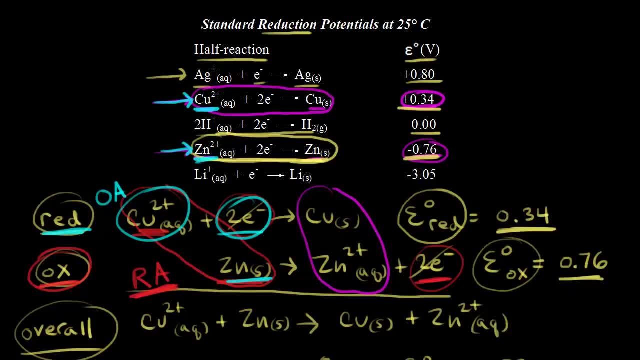 to zinc two plus ions, right. Well, copper two plus, we know, is more easily reduced, right. It has the higher, has the more positive value, I should say, for the standard reduction potential. So copper two plus is more easily reduced. 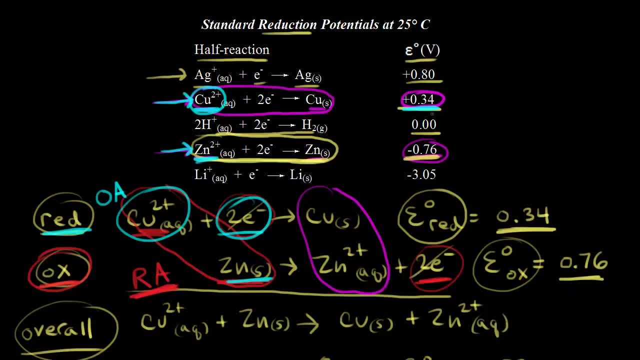 And therefore copper two plus is a stronger oxidizing agent than zinc two plus. So as you go up on your standard reduction potential, you're increasing in the tendency for something to be reduced And therefore you're increasing the strength as an oxidizing agent. 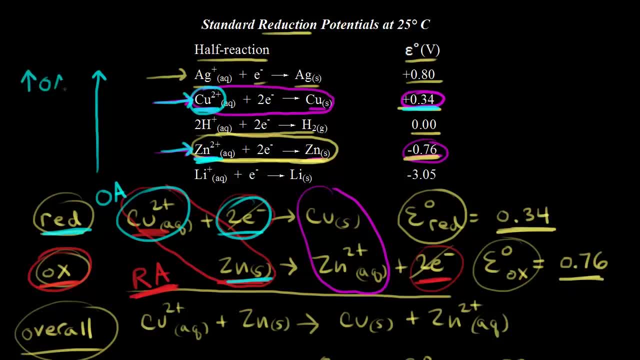 So as you move up on your standard reduction potential, increased strength as an oxidizing agent. So copper two plus is a stronger oxidizing agent than zinc two plus, All right, So let's think about the opposite. So as you move down on your reduction potential, 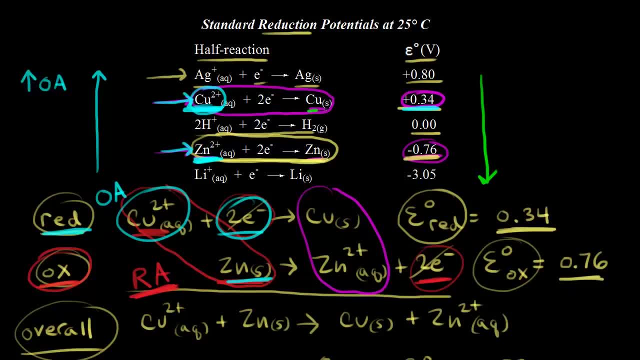 So as you move down here, So let's compare solid copper and solid zinc. right, We know that solid zinc was our reducing agent in our reaction, And that's because the reduction potential was the more negative one. So that means this is more likely to be.